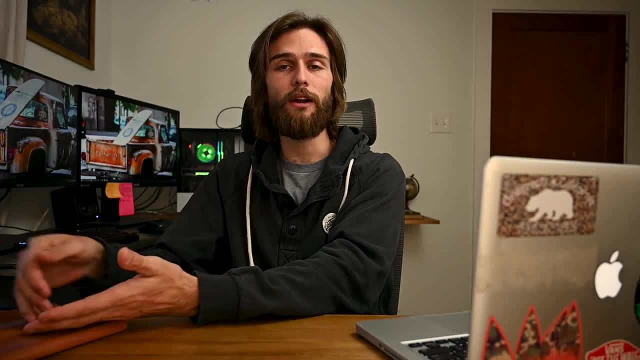 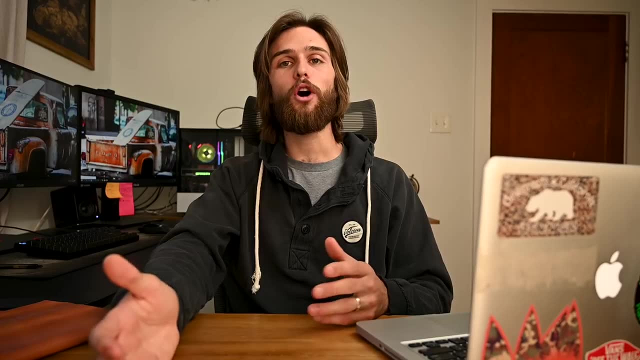 software and you're effectively working fresh on whatever you're working on next sprint. That way, you're not going to be very adverse to any changes that come along the way. Now, what I personally do and what I typically talk about on this channel, I would consider scrum, which scrum is a type 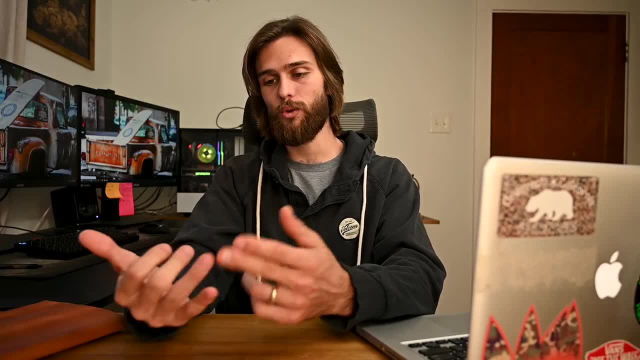 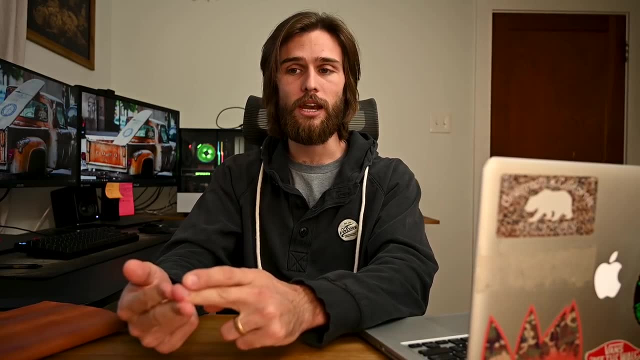 of agile methodology, but there are plenty others, like Crystal. Lean- kind of sounds like I'm listing drugs right now, but I swear I'm not- Kanban, which a lot of times is a subset of Lean, and many more. While they all follow the same principles of agile development, they each have 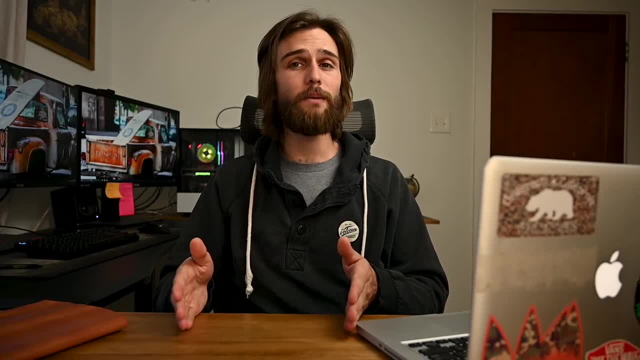 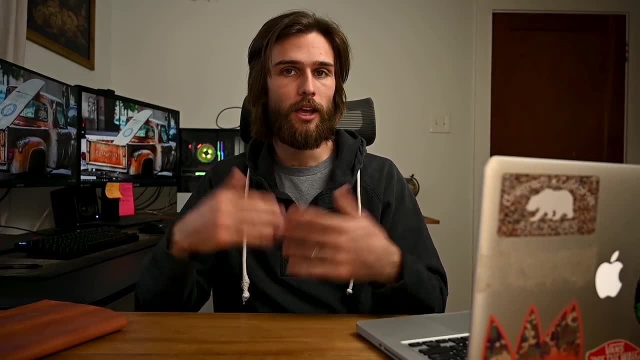 their own twist on it. This isn't the video where we go into depth on the types of agile development, just talking about the overall details and principles of agile development itself. So if you wish to do more research, look up types of agile development and go from there. 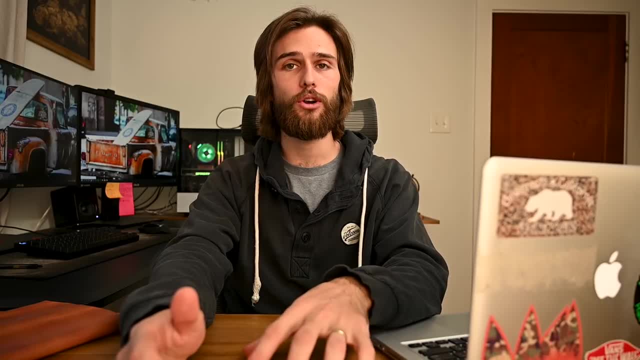 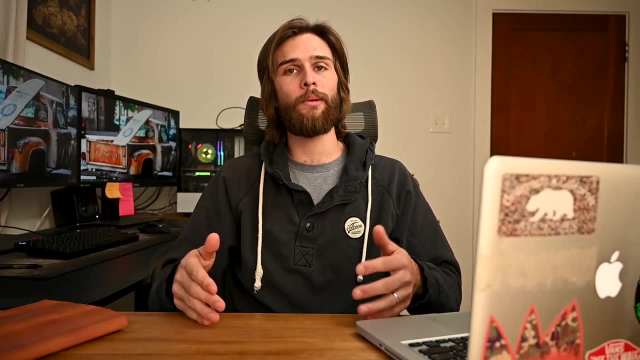 To help you avoid confusion, I recommend not doing that because, just like when you're learning programming fundamentals, it makes it a lot easier to learn different languages because you already understand how programming languages work. It's just a matter of learning syntax. Same thing goes. 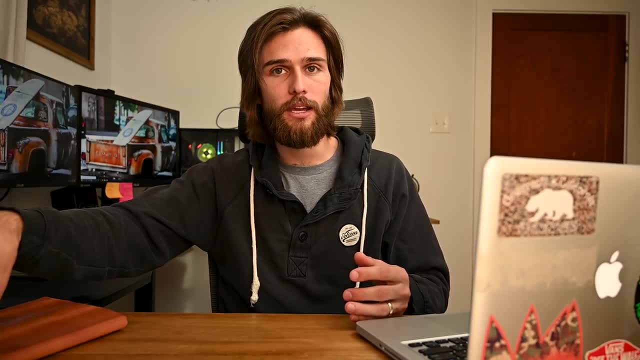 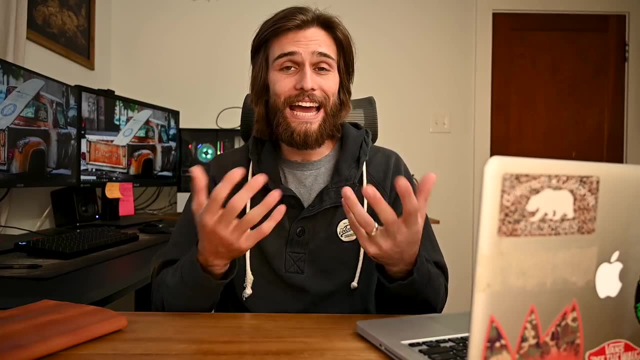 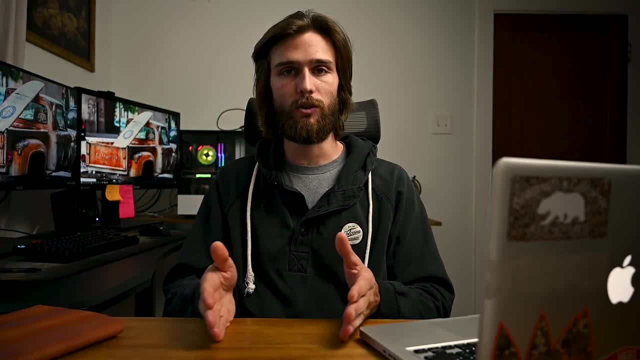 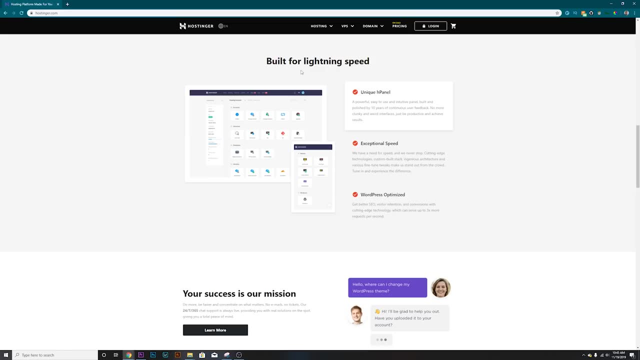 Watching this. our web developers are aspiring web developers, And what are you going to do after you follow the agile methodologies in creating your website? Well, you're going to have to find a web hosting provider, Whatever web hosting you may need, whether that be shared web. 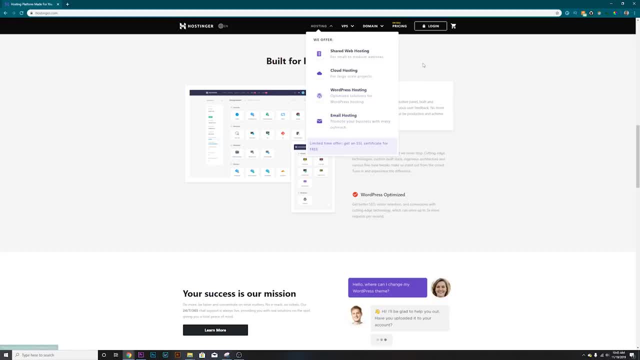 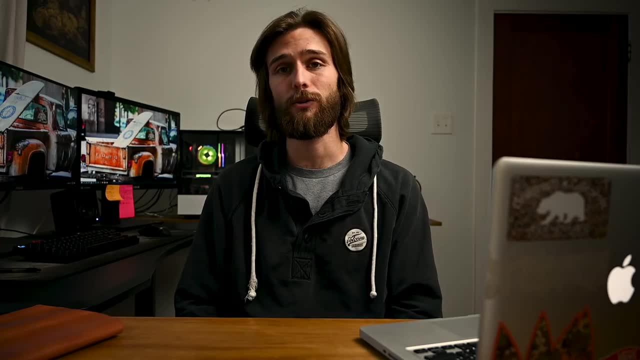 hosting, cloud hosting, WordPress hosting, email hosting, VPS hosting. Hostinger has it all. They also offer free SSL certificates. They have a free site builder in case you wanted to go there. I know a lot of y'all work on WordPress and Hostinger fully supports WordPress. 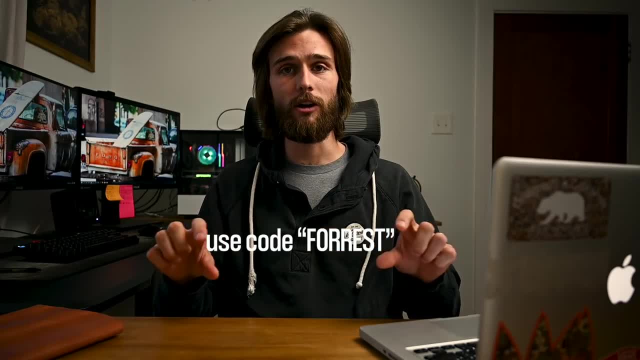 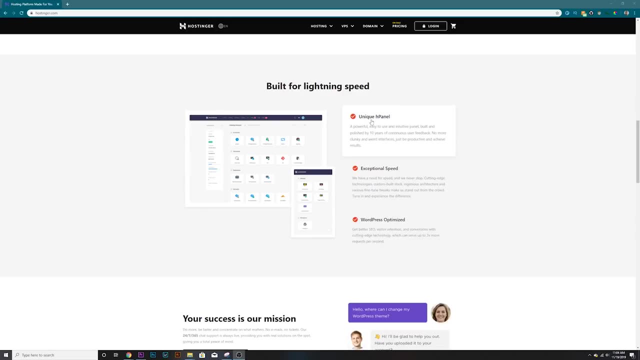 blogs and sites. And something even cooler is that, when using promo code Forrest with Hostinger, you're able to get 91% off for their Black Friday sale And within Hostinger, you're able to access your cPanel. This is just a full-on one-stop shop for whatever you need in terms of web hosting. 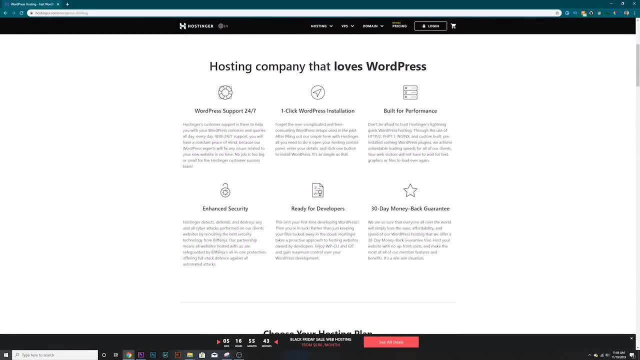 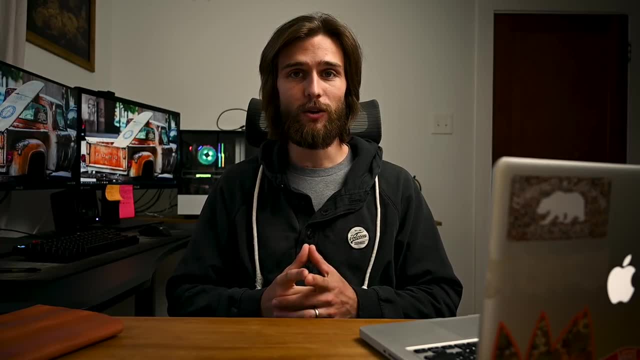 domain registration. what have you So? I'd really appreciate it if you showed your support. Use the link in the top of the description, Sign up for Hostinger And remember 91% off for their Black Friday sale when using code Forrest. All right, So the best way for me to explain this, as always, 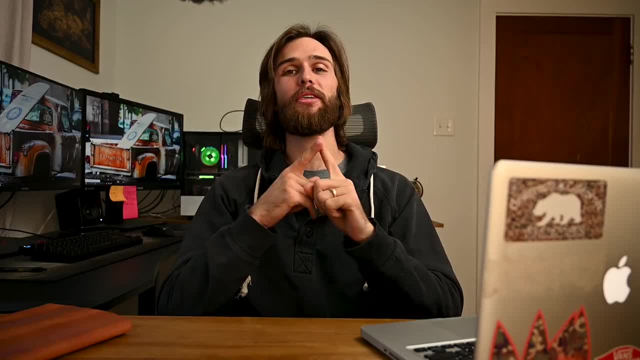 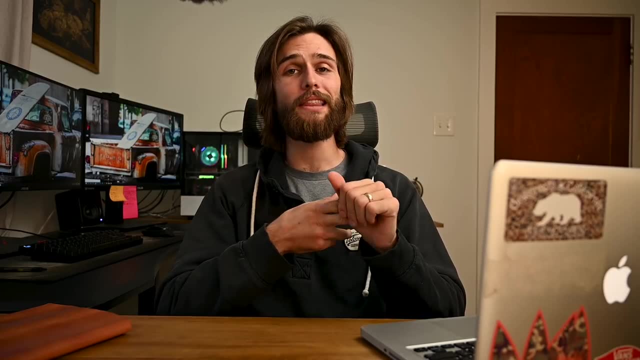 with an analogical example When I was remodeling this house. it really got me thinking about one day building the dream home, a big house to fit a big family. But in order to do that, you'd have to save up a lot of money, buy the lot and build this house. That's how most people do it. In all, 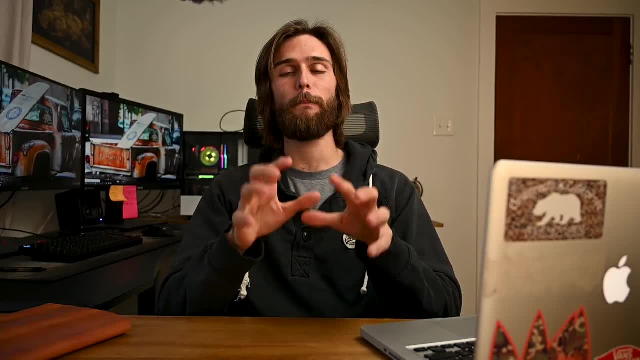 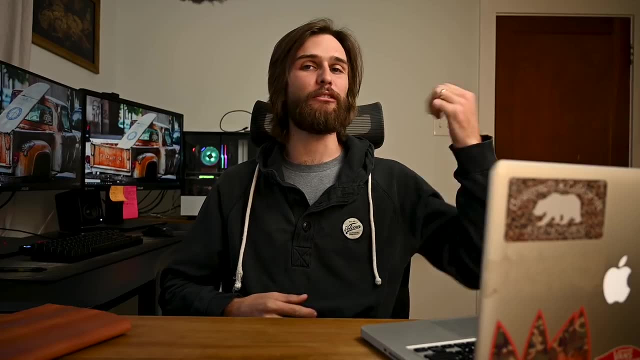 honesty. that's kind of how I plan to do it as well. But for the sake of comparing this to building software with agile development, let's pretend that's not my plan. Let's pretend my wife and I get evicted from this house. We get a 90-day notice. Get your stuff out. Get out, Buy 90. 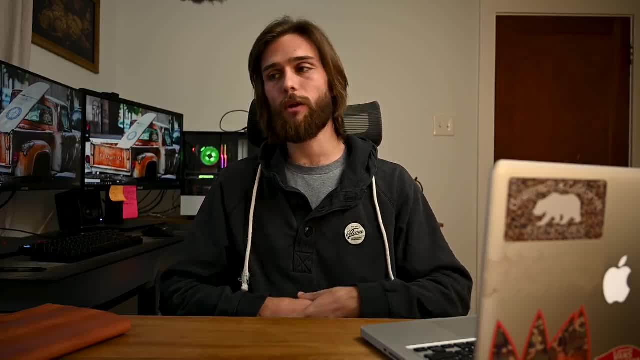 days Done. Well, you know where we are in our lives. we don't want to go back and live with our parents. We don't want to get evicted again, so we're not going to go rent somewhere else. So the 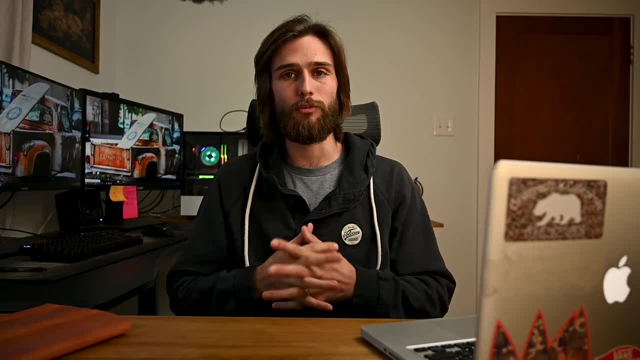 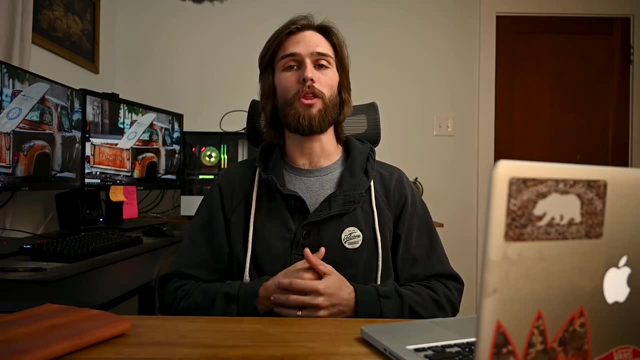 only real option is to go and buy a lot and build a house. But we can't afford to build a big house. We don't even have enough time to build a big house. So what do we do? Well, instead of building the big dream home all at once, you build it in smaller iterations. You start off with the heart. 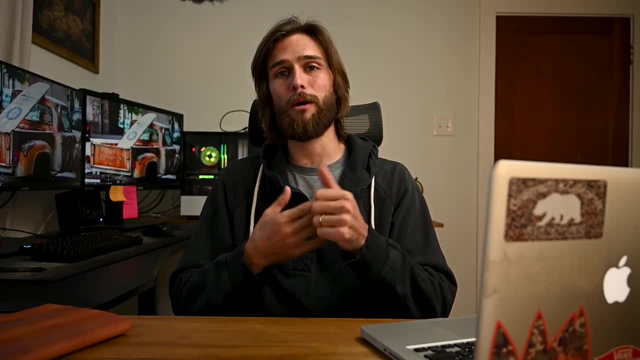 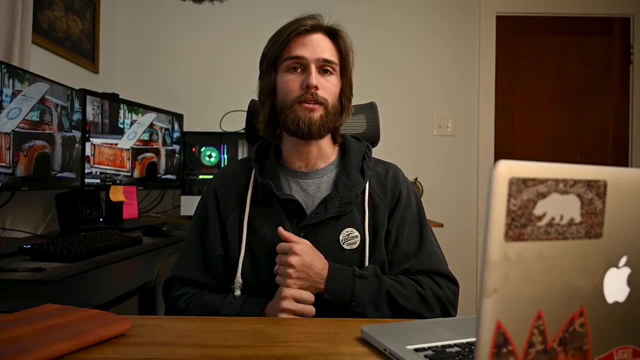 of the home. You have a kitchen, a living room, a bedroom, a bathroom and maybe a closet. if you're have to have a closet in order for it to be considered a bedroom, So that has to be included as well. This house is perfectly livable. You're there for a couple months. You're saving up a 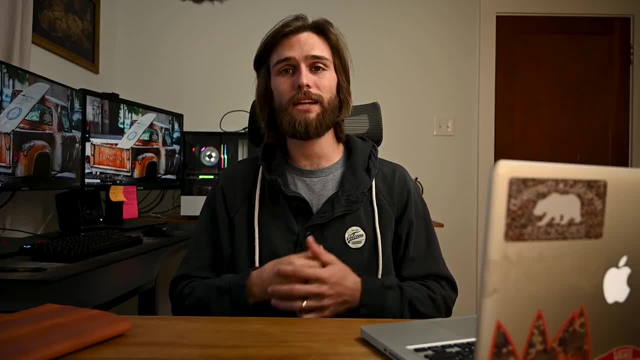 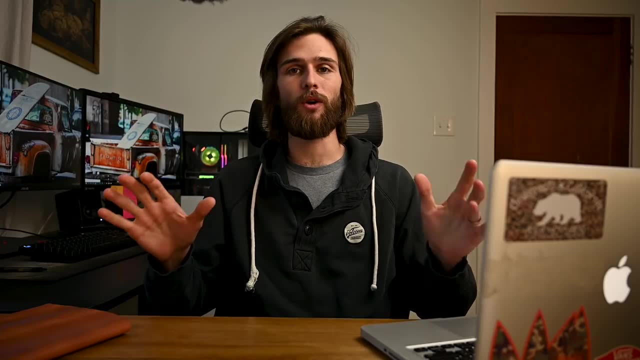 little bit more money and then boom, you have a kid on the way. Now you need to expand. so you build another room. It's perfectly enclosed, It's perfectly livable. But then your job changes. They decided they're not going to have any on-campus work, They're going to do everything remote. So 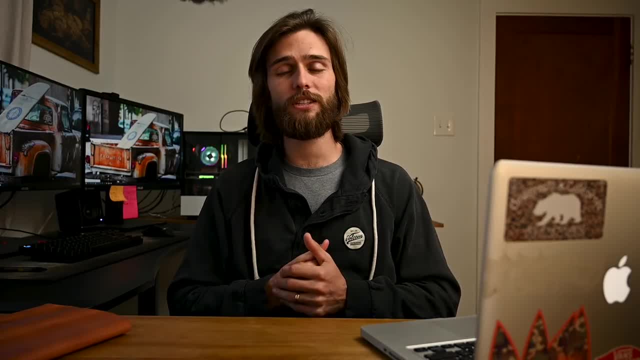 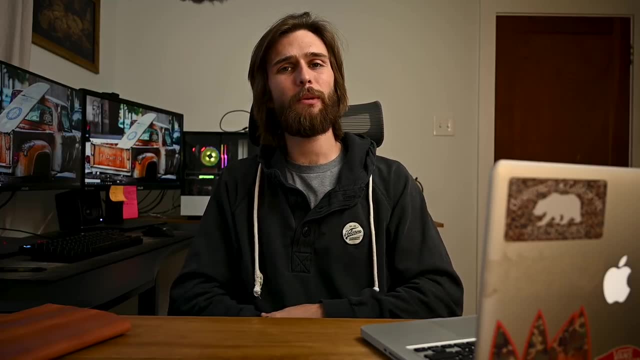 now you need a home office, so you add that on, And then, for whatever reason you decide, you want to build another bedroom. add another bedroom onto the house, but you also realize that you don't really like the bedroom you're currently staying in- The bathroom isn't? 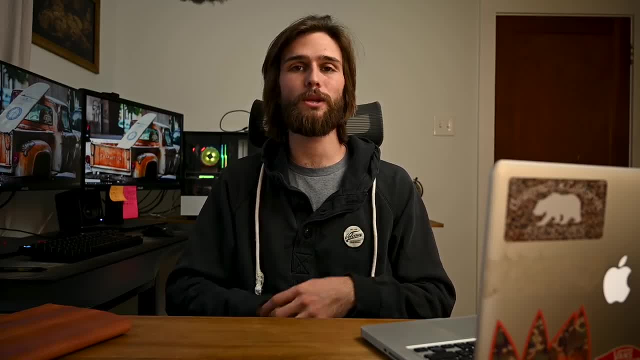 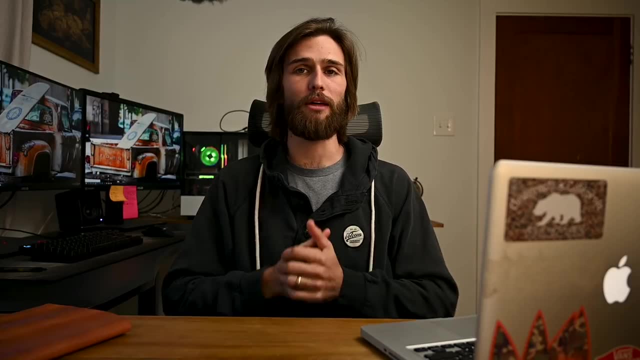 connected to the bedroom. so you have no en-suite And the bedroom's a little bit small, The closet's a little bit small. So you want a proper master suite, Big room, walk-in closet, nice bathroom. So what do you do? You make the old bedroom into an office new bedroom that you're going. 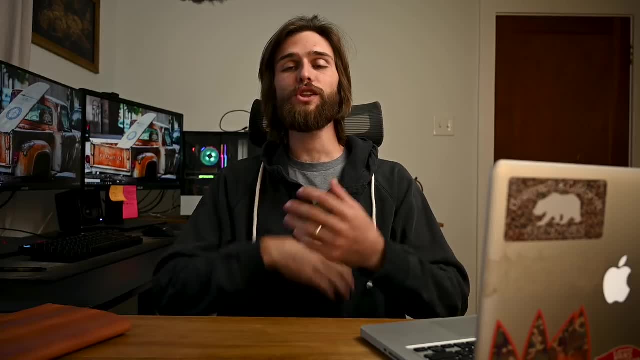 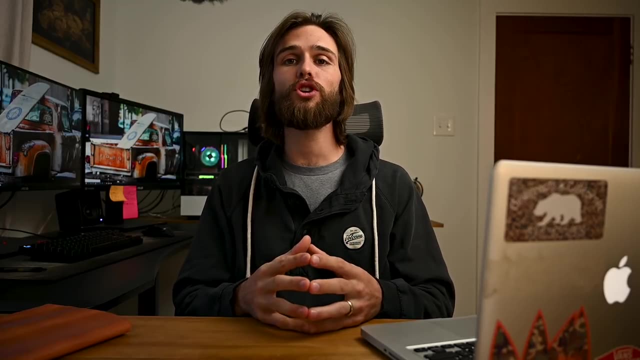 to build anyway, and you build yourself new master suite And then you keep adding on until you finally have the house of your dreams. And that's the kicker with Agile development: Just as you start off with a small, livable house, you start off with small working. 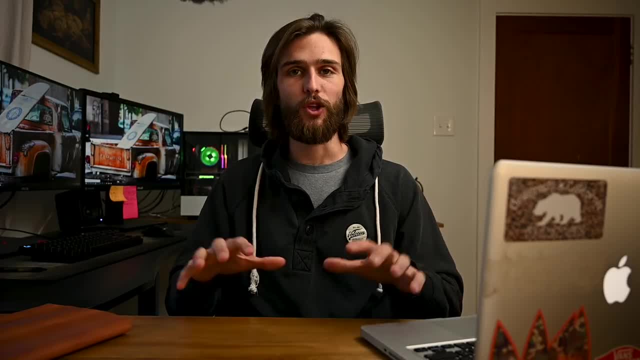 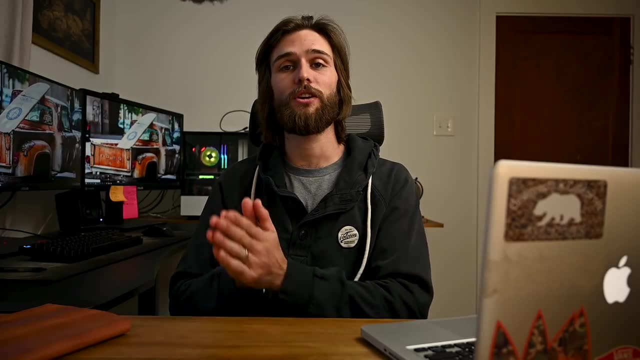 software. Just as you add on completed rooms to your house, you add on deliverable features to your software. Just as you made an adjustment to your plans by building a master suite instead of just another bedroom, you can make adjustments to whatever feature you need to implement. next, 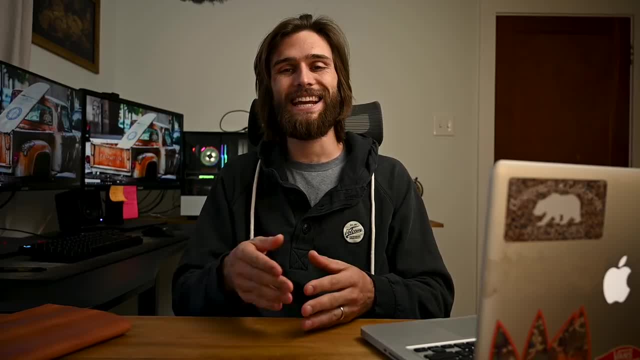 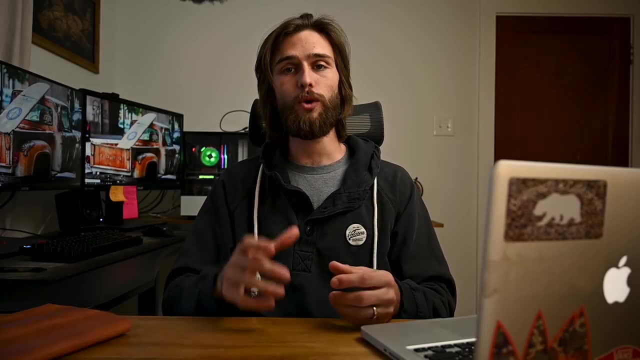 Well, if you follow the waterfall method, which is popular in its own right, each section of work would depend on the previous section of work. Just like if you decide to build a big house at once, you can't move in until the drywall is up. You can't put up the drywall until 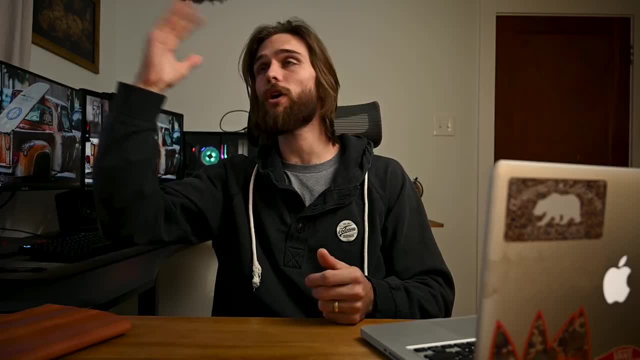 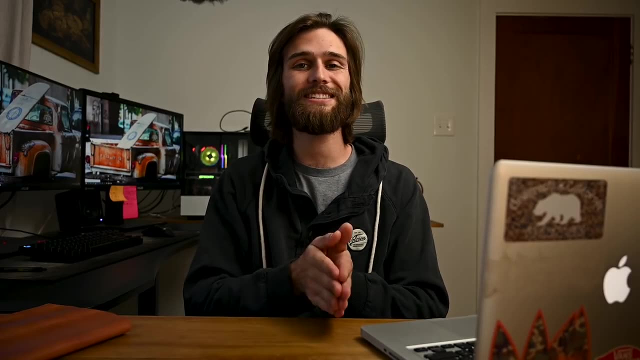 the installation is in. You can't put the installation in until the walls are up And you can't put the walls up until the foundation is set. Sure, this goes for the smaller house as well, but the difference is size. For the smaller house, it could take you a month to build, while the bigger house it'll take you six months to build. You're able to move in after a month instead of after six months. It's just like building smaller software and adding on to it. You can give your client a product, a working, simple software after a month and make any additions. 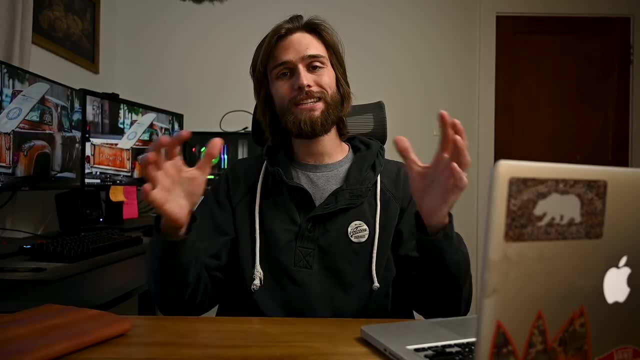 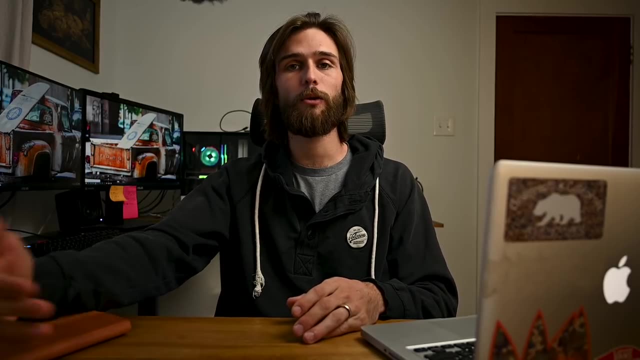 or adjustments you wish over the next five months, While if you decide to build the entire project at once using the waterfall method, well then the client will be able to see that for another six months They won't be able to make any adjustments until thereafter, Meaning if the priorities change. 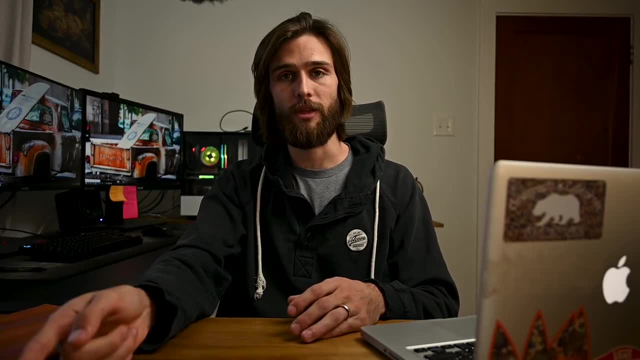 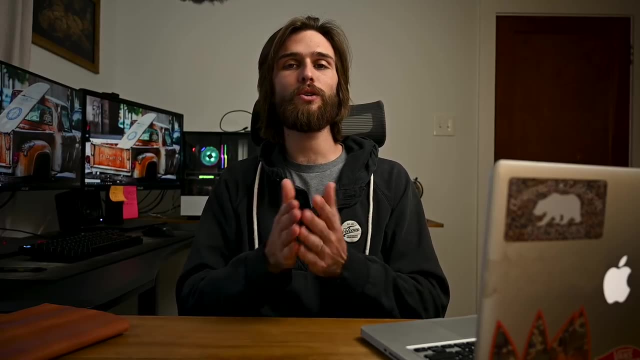 or if they don't like something, you're going to have to spend extra time there working on whatever they need done. At least, that's the best way I understand it. Now that you understand agile development, how does it work in real life on a real project? Let me take you through that. 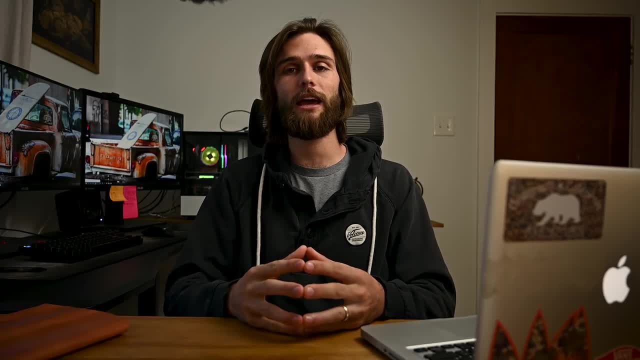 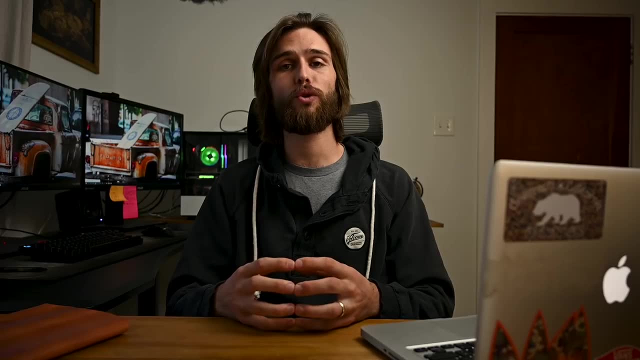 You have an application you need to build and your team takes time to break that application into user stories, That is, smaller chunks, features that you want to implement, user stories. Then they break those user stories down into tasks, all of which is located in your backlog of whatever. 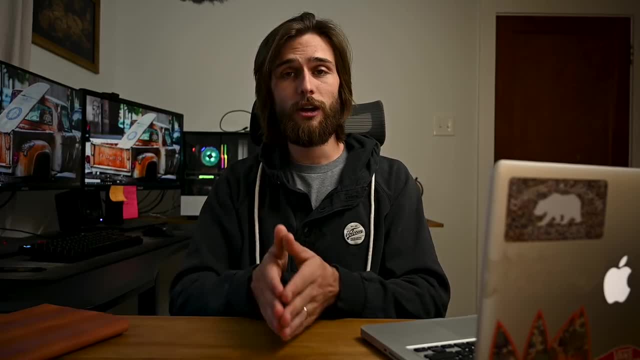 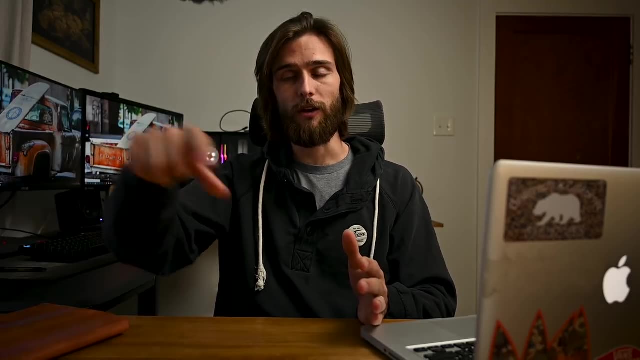 project management software you decide to use. Then you're able to create a sprint: two, three, four, week, whatever it may be. You take those tasks and user stories. whatever you need to get done in this sprint, you drag that over based on the prioritization set by. 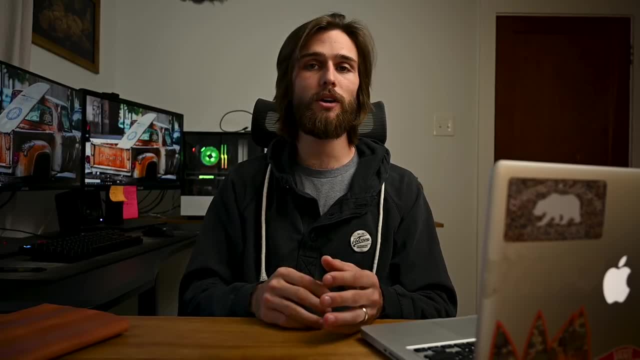 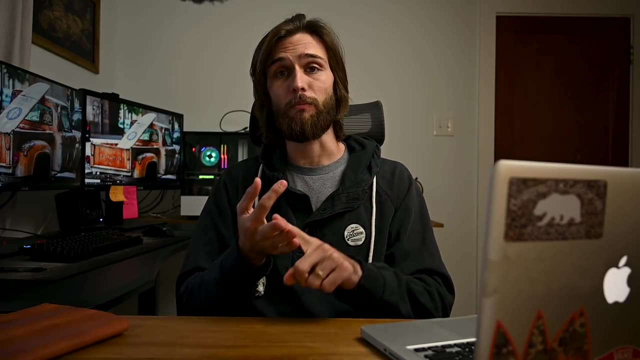 your project manager or the client And each day, during the sprint, you come into work, you pick your task for the day. you go into standup, you talk about what you did yesterday, what you're going to do today, any impediments, and then you get to work. You get done with that task. 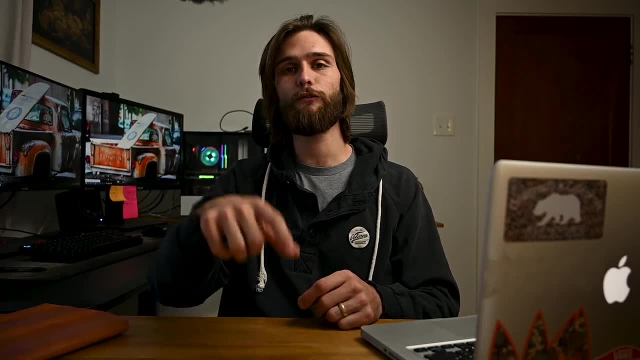 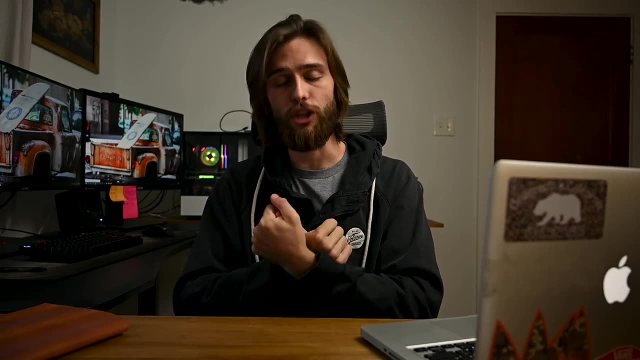 you pull on another and you complete that one, And then you pick up another task when you fully complete that task- That means code test, successful build, pushed, submit it for peer review- and then you go on to the next task, And then you go on to the next task And then you go. 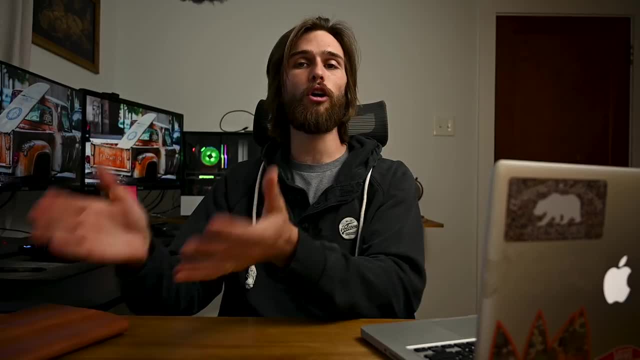 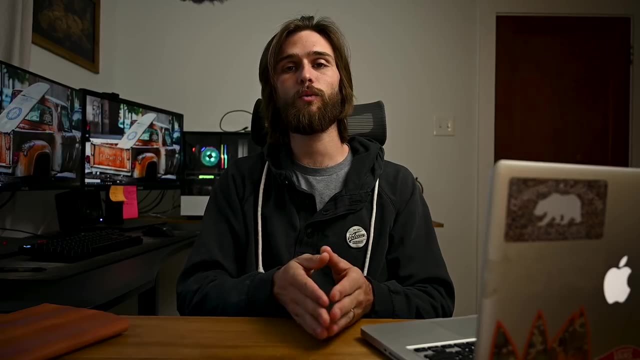 on to the next task. You do this every day until the sprint is over, And now all of that code is over in QA, quality assurance. And then you have a meeting with your team, your project manager, maybe even the client, to determine what you need to get done. the next sprint, The next sprint is: 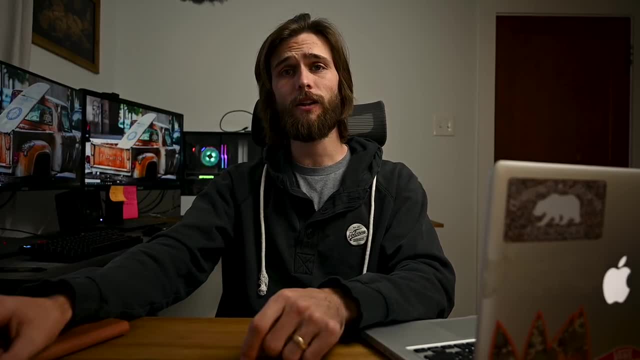 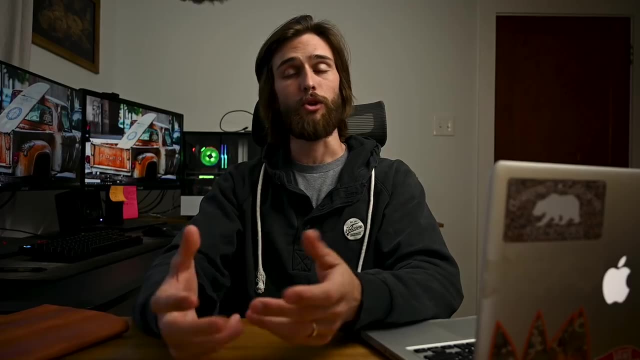 basically the same, but you may find yourself adding more tasks to the backlog because you're gathering information from the QA testers that you'll need to get done either at the end of this sprint or next sprint, And then you repeat this cycle, with minor variations for each sprint. 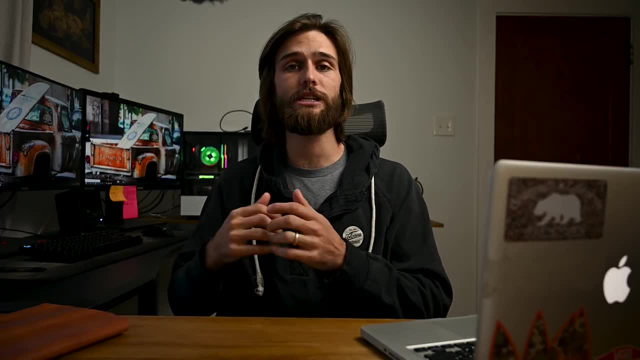 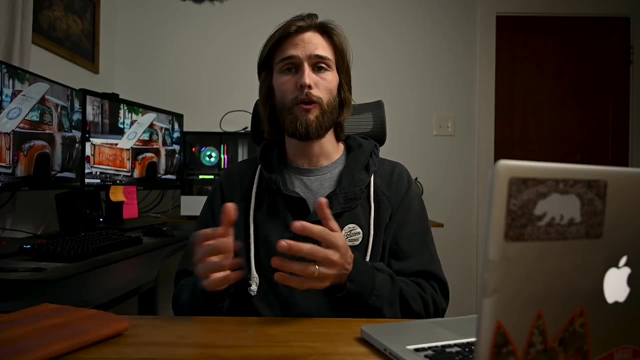 I've actually made an entire video about how to go about completing a software engineering task, where I take you inside Jira, a project management tool. So if you want a more in-depth look at how to go about completing an actual task, I'll link that up in the card above. That is it for today. Don't forget to show your support. 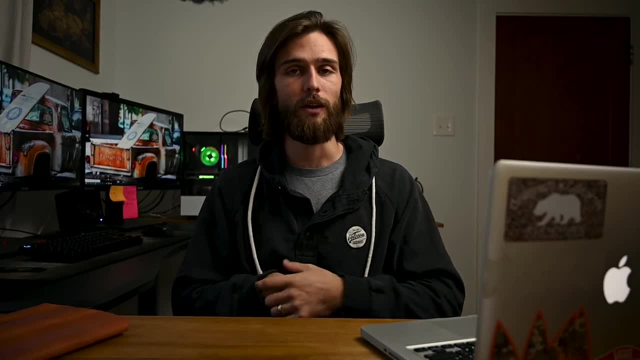 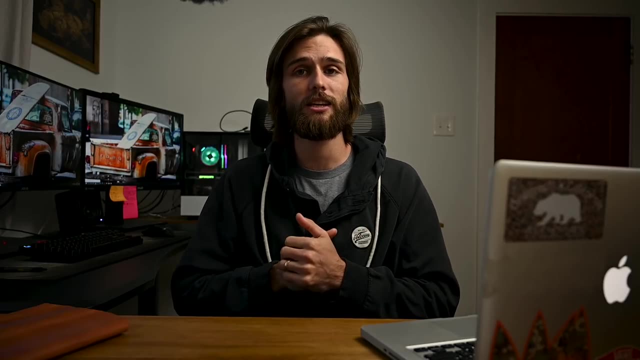 check out Hostinger with the link I left in the top of the description. If you liked this video, give it a big thumbs up. Any questions, leave those in the comment section below. Consider subscribing if you like videos like this, and I'll see you on the next one. Have a great day.